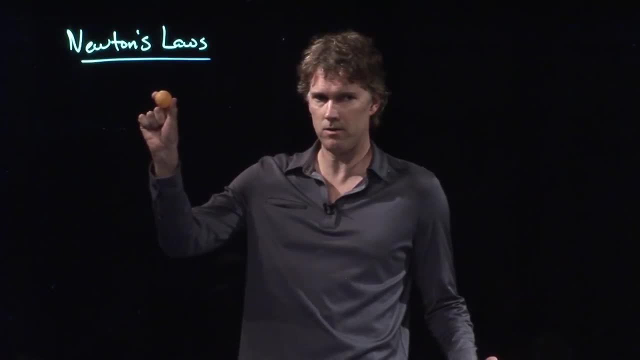 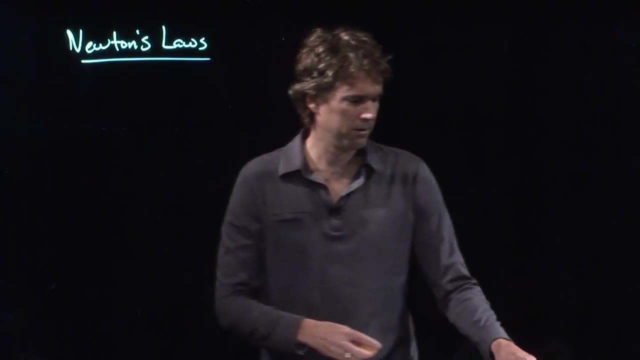 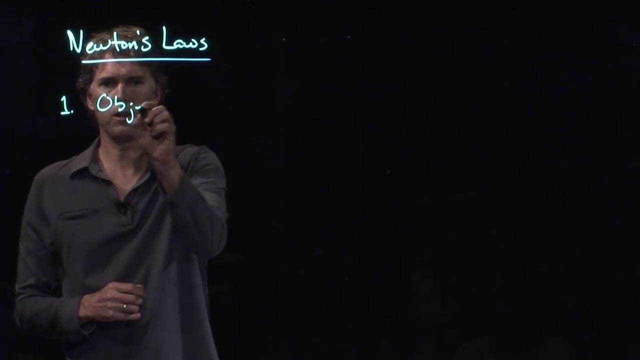 It started at rest, It's in my hand And in fact, right now this thing is still at rest. right, It is not in motion. And this is Newton's first law. okay, He had three, and the first one is: objects at rest tend to stay at rest. 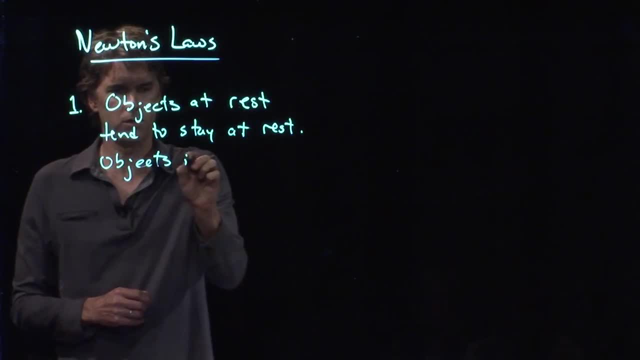 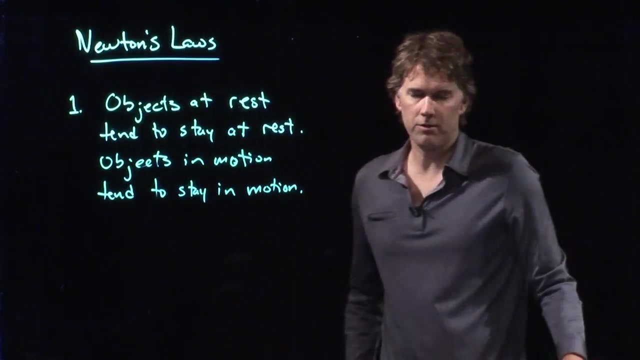 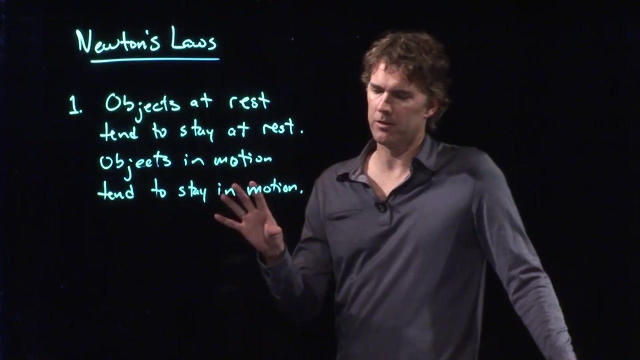 Objects in motion tend to stay in motion, And this sounds rather intuitive now, but when Newton came up with these laws, they were rather counterintuitive. So let's just think about this for a second. Objects at rest tend to stay at rest. okay, Here's a. 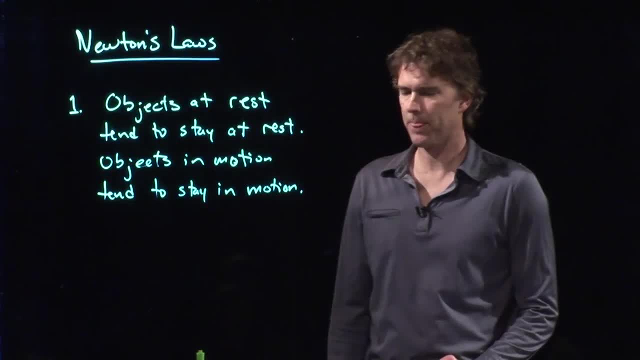 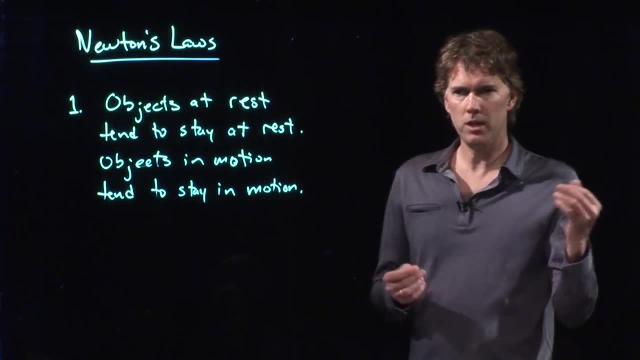 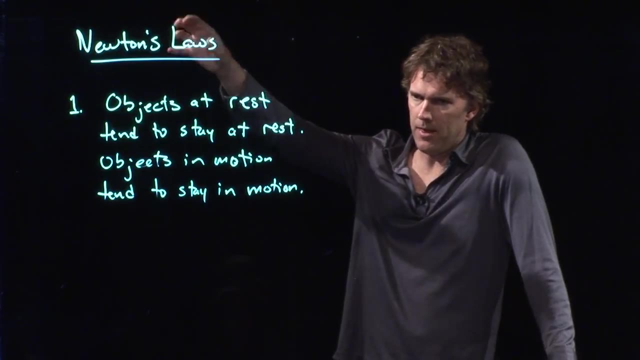 pen. I put the pen on the table, You can see the cap there And it's staying at rest. If I throw the pen, it's in motion. It's tending to stay in motion And in fact that object, when we were holding it it was at rest And then it started moving. 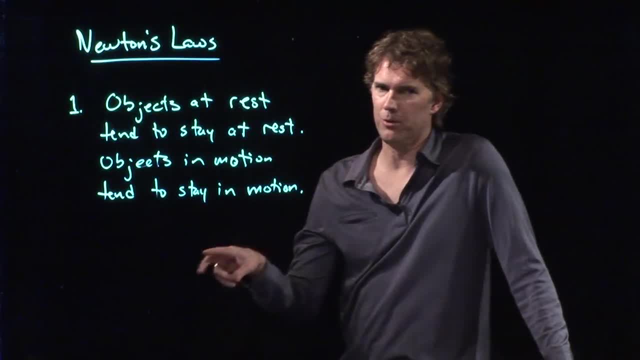 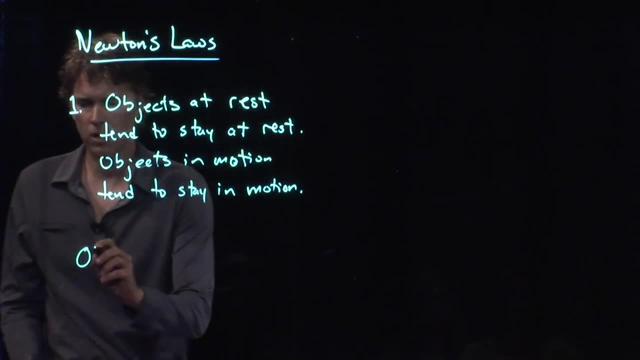 It started accelerating, As we're going to see in a second. that's really Newton's second law, because it's dealing with acceleration. But if we think about, maybe, Olympic curling- I know that's all you're familiar with, I know that's all you're familiar with, But 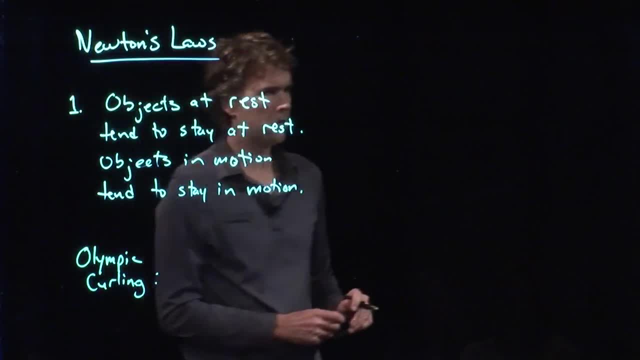 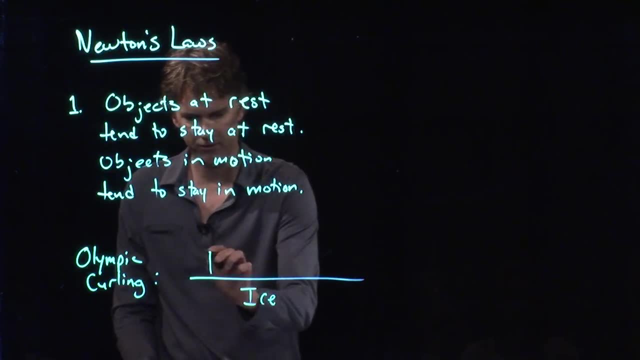 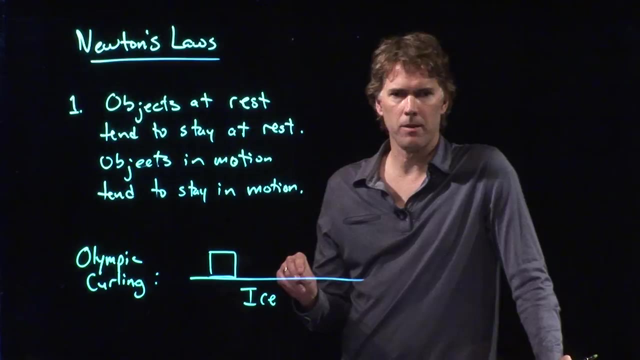 it's just one of your favorite sport out there, right? Olympic curling. What does that look like? Well, here's the ice, right, And you have this stone which comes from a particular, a particular island in Scotland, which is where they make these stones. There's. 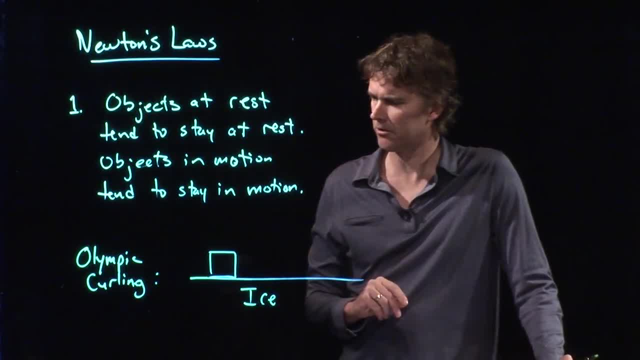 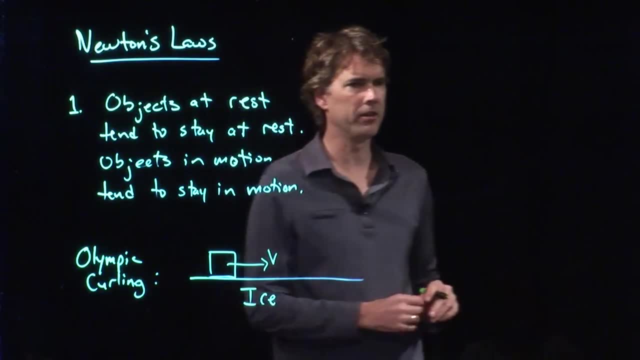 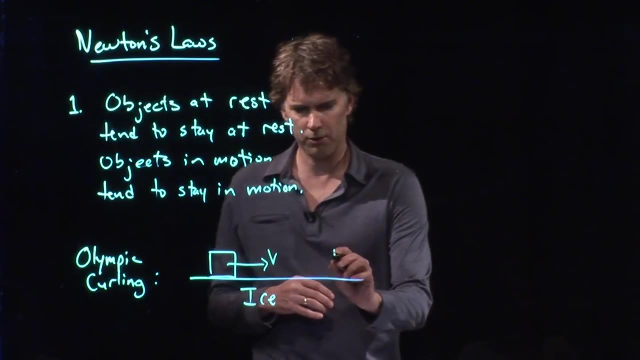 only one place in the world where they make these stones, which is kind of strange. But curling itself is kind of strange, so why not? If that thing is moving along at velocity v- And I think about this object at a later time when it's over here- How fast is it moving? 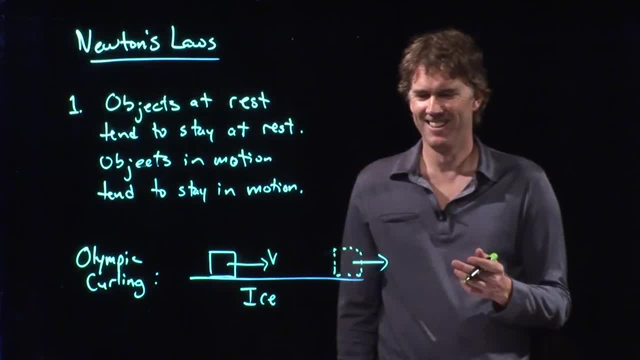 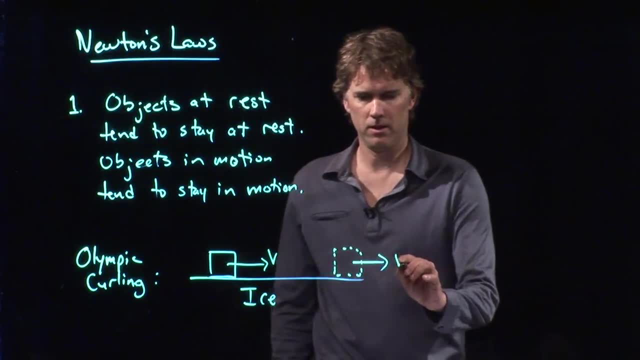 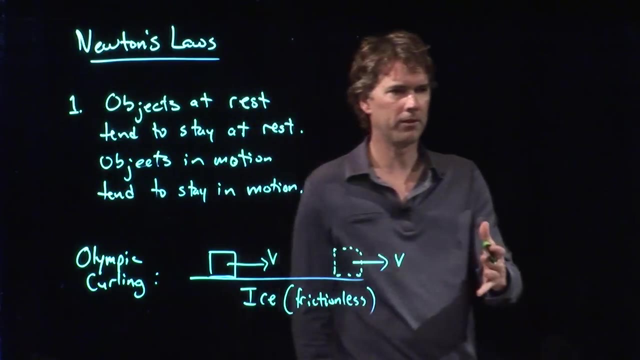 along at roughly Megan. what do you think? What speed is it moving at later? on The same speed that it started moving at? Aha, No friction. Yeah, If this is nearly frictionless, then it will be moving at the same speed. 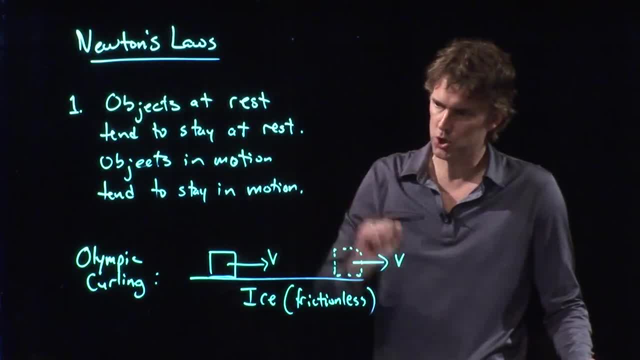 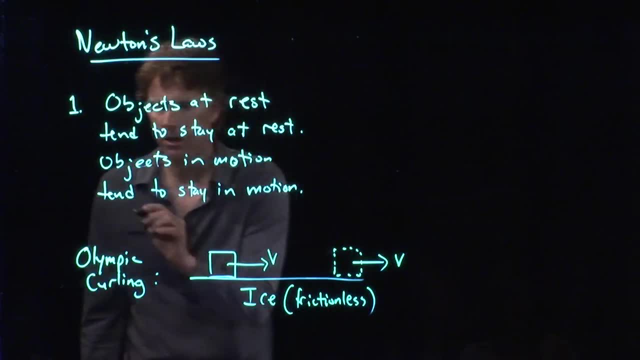 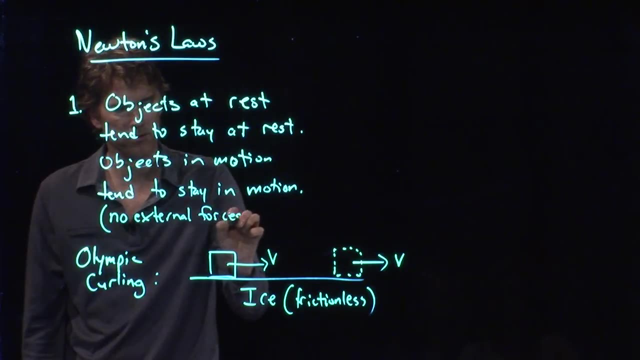 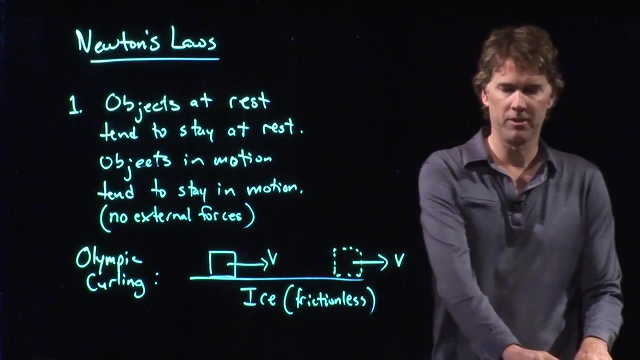 And that's Newton's first law: Objects in motion tend to stay in motion, And so, really, what we should put is this little caveat- We can put this here: No external forces. Okay, There's nothing that's trying to slow it down, There's nothing that's trying to speed it up. Obviously, in the 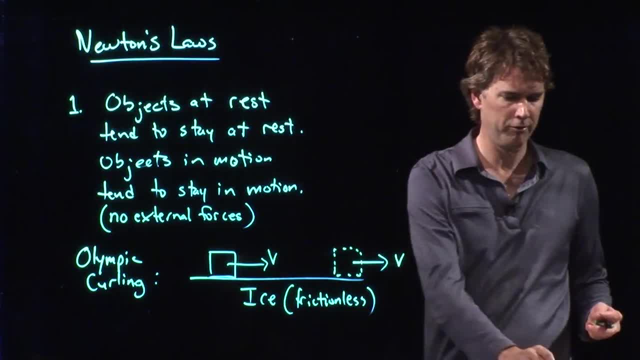 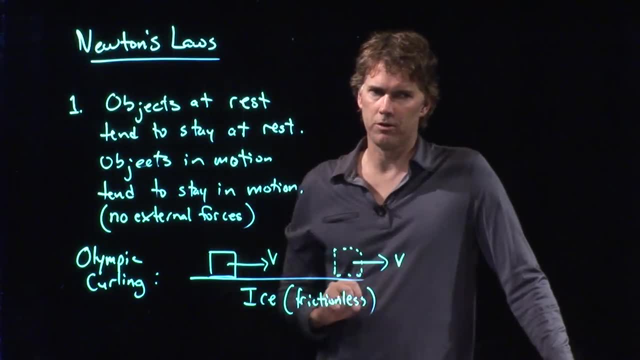 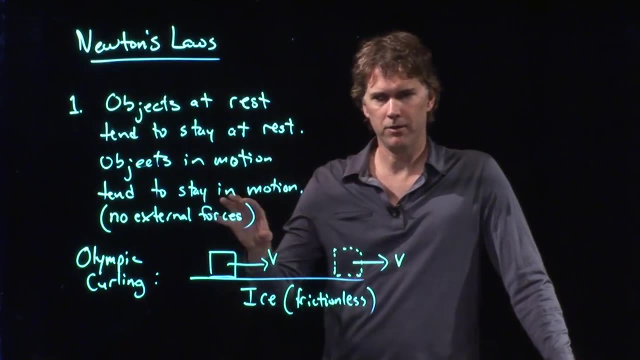 example of the ping pong ball dropping, we do have an external force. We have gravity that is trying to pull it down. So Newton's first law is really: no external forces. Objects in motion tend to stay in motion. If I put that stone on the ice and I just leave it there, 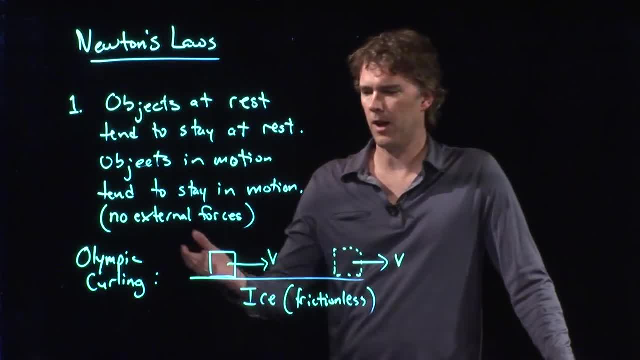 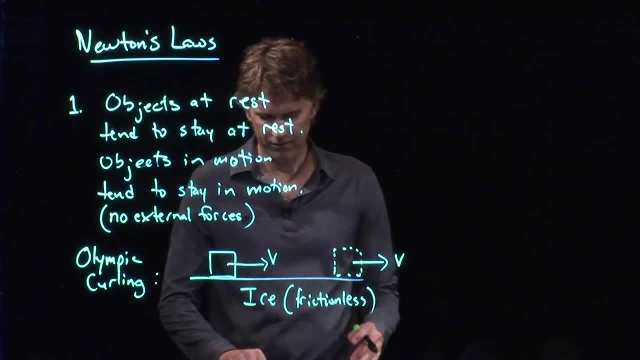 at rest. it will stay there at rest. If I push it and it gets velocity v, then it will keep velocity v for a long time, All right, So that's Newton's first law. And one way to think about Newton's first law is: 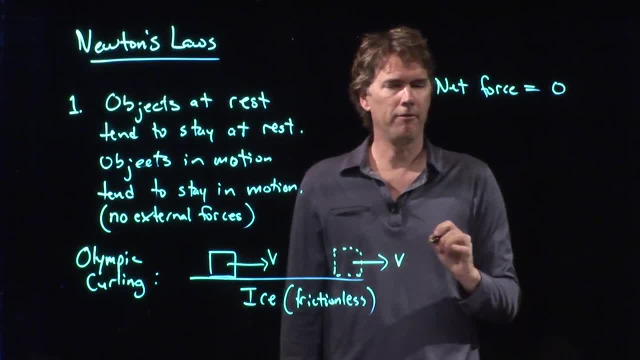 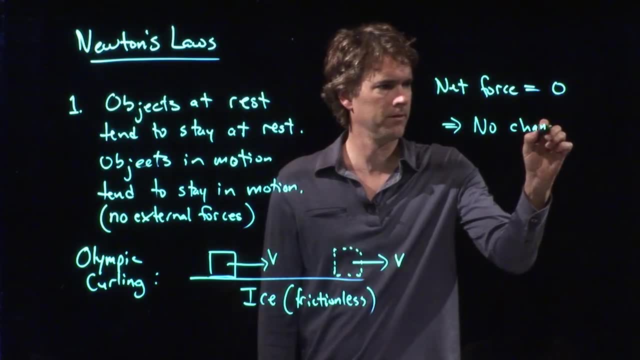 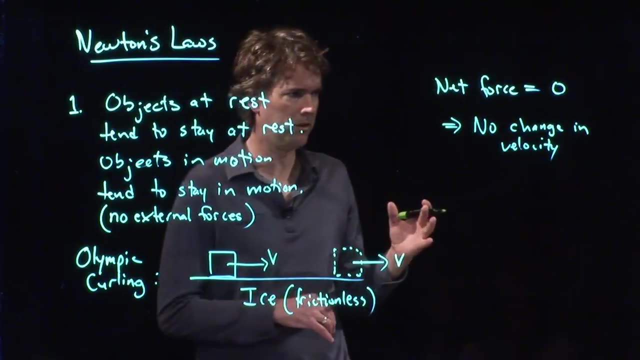 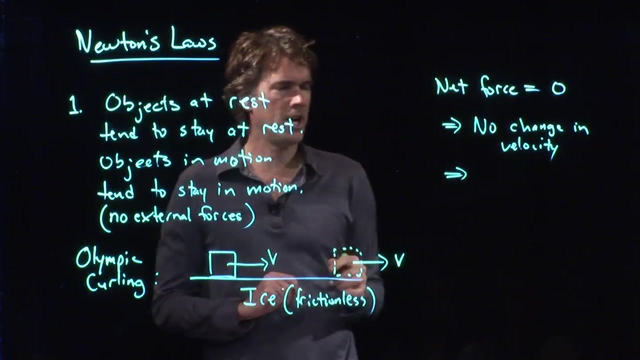 is this: The net force is equal to zero And therefore there is no change in the velocity. That velocity could be zero and at a later time it would still be zero. Or it could be some value and at a later time it would still be that value, But we know exactly what change in velocity is. 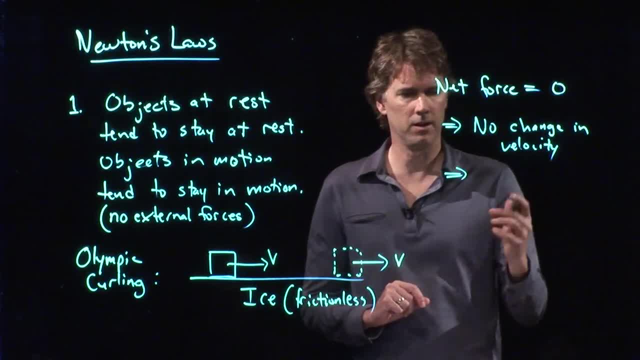 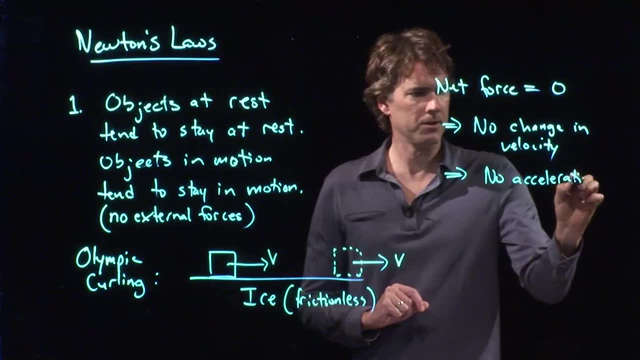 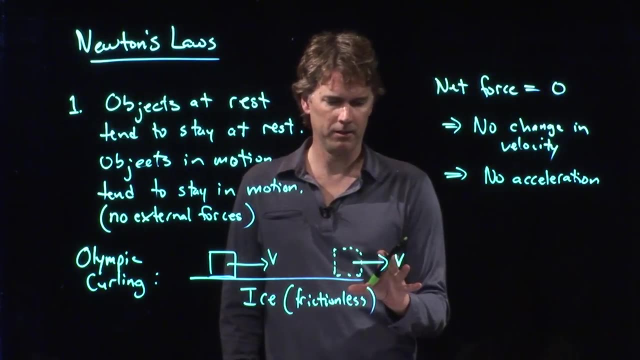 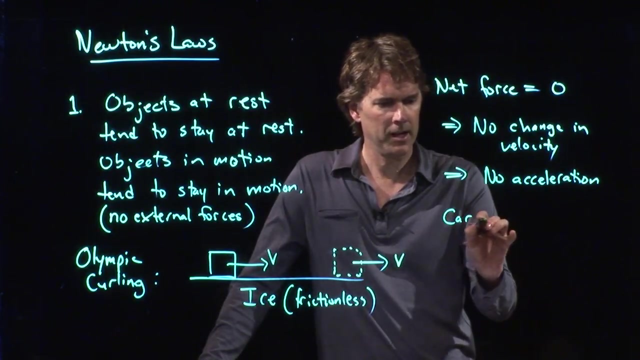 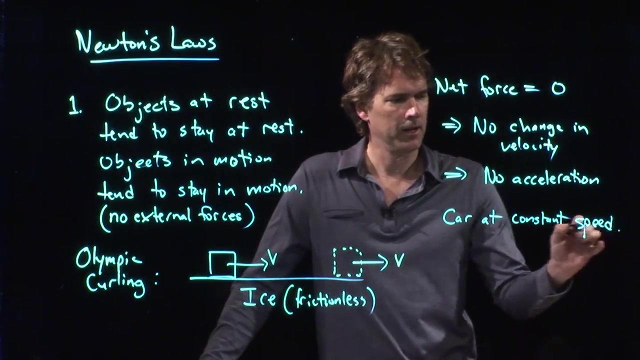 Change in velocity is acceleration. All right, A is delta v over delta t, So this must mean that there is no acceleration. Okay, This is already a little perplexing to people, because let's say you're doing the following experiment. Let's say you're driving down the road in your car at a constant speed, in a straight line. 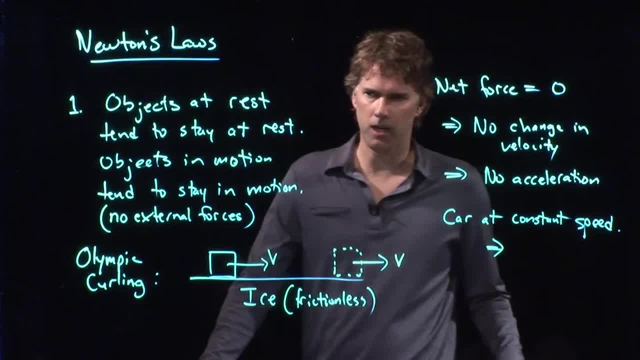 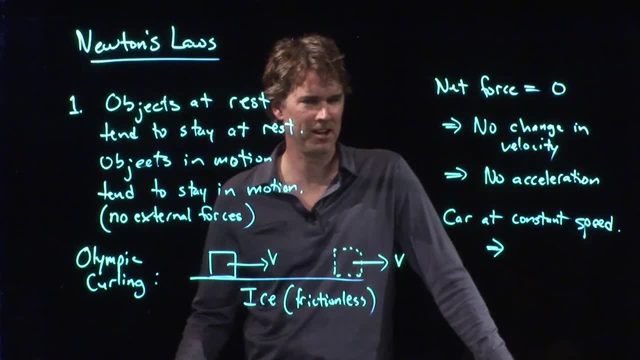 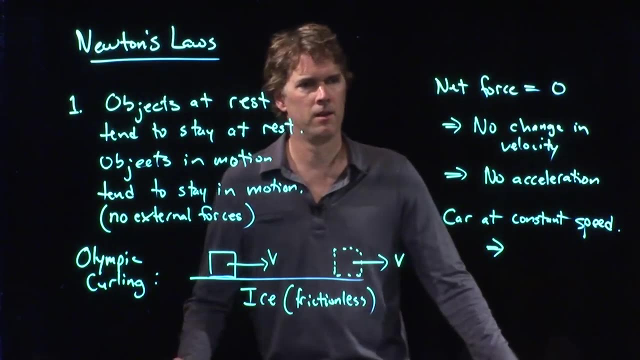 Is there any acceleration for that vehicle Stacy? what do you think? Is there any acceleration if I'm driving my car at constant speed in a straight line? No, because it's in constant speed, That's right, Because it's constant speed and it's a straight line. 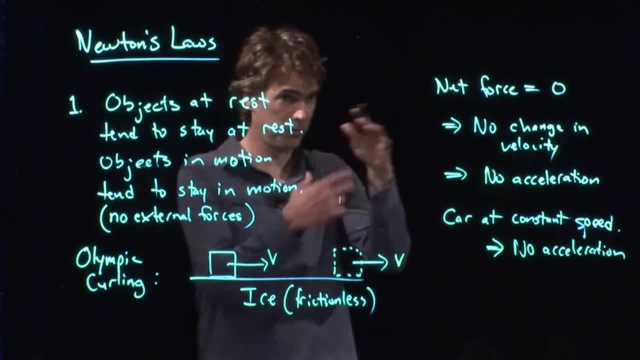 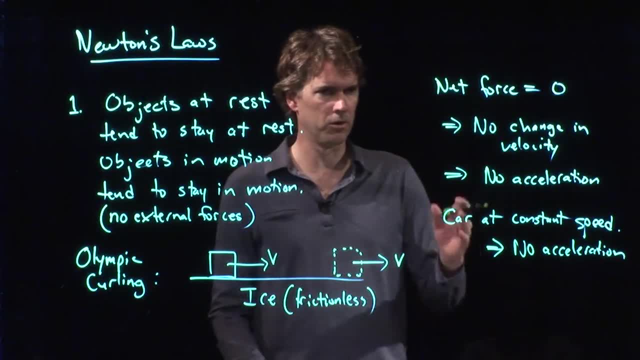 As we learned, if I'm driving at constant speed, but I'm driving in a circle, then there is, of course, acceleration Right Going towards the middle. Exactly, It's a centripetal acceleration towards the center of the circle.